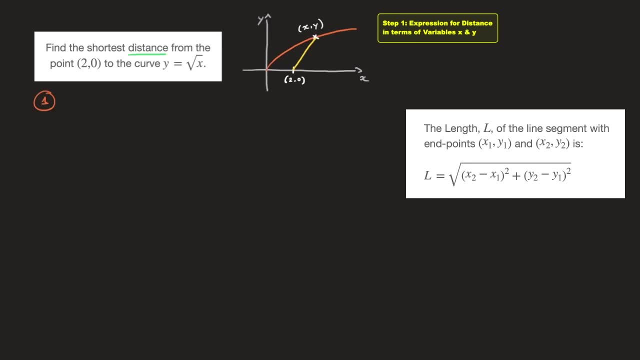 And we've already seen the formula for the length of a line segment with endpoints x1, y1 and x2, y2.. Indeed, that's the one we see right here, And so, using that, we can state that the length of this yellow line segment, which I'll go ahead and call a d for distance, is equal to the square. 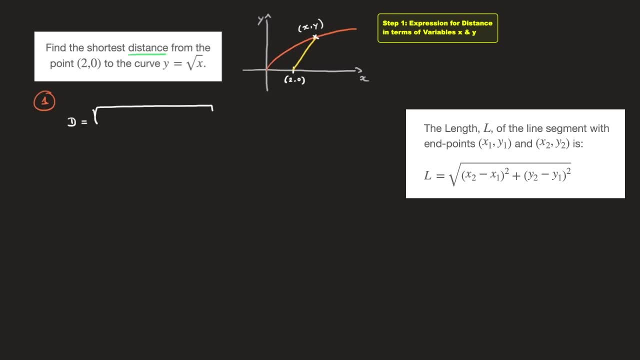 root, and I'll just make a large square root here. there we go, of x minus 2, all of which is squared. So I'll write that that's x minus 2, in parentheses, squared plus y minus 0.. And again, 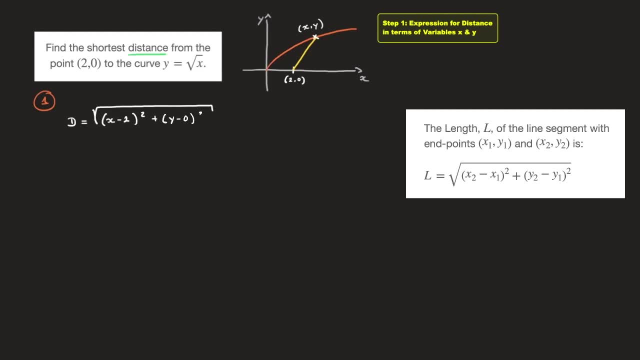 that's squared. so I'll write that in parentheses: y minus 0 squared. Now, opening up each of these two pairs of parentheses leads to: d is equal to the square root of x minus 2 squared, which is x squared minus 4x plus 4, plus y minus 0 squared, which is just y squared, And that's our. 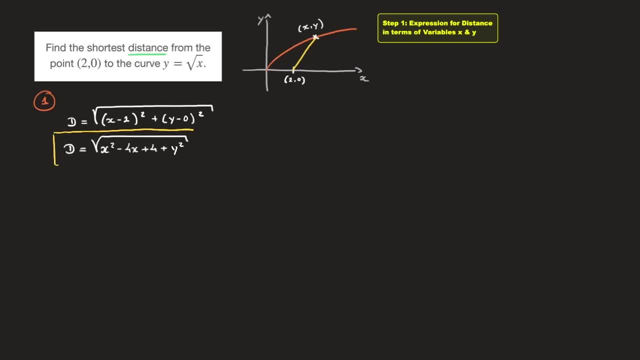 first step done, We now have an expression for the quantity we're trying to optimize in terms of the variables x and y. So we move on to step two, And in step two we need to find or identify the constraint and make sure that it's written in terms of the same variables as 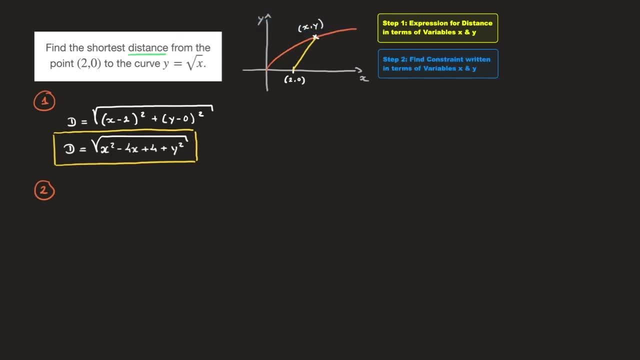 the expression we just wrote. In other words, we need to make sure that it's written in terms of x and y, And when I say constraint, you could go ahead and ask yourself what's the limitation here. In this case, we're trying to make the distance from the point with coordinates to 0 as short as 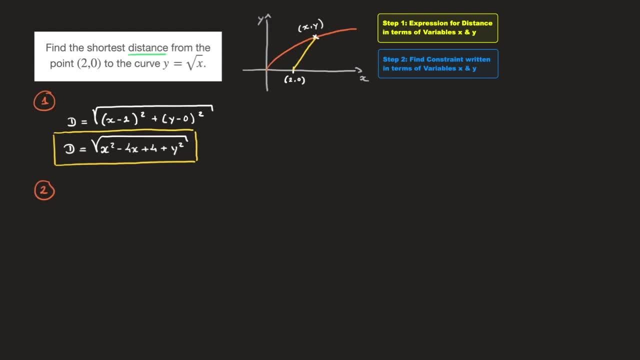 possible. So what's stopping us from making it 0?? And we quickly find that the only constraint or limitation is the fact that the point has to lie on the curve. y equals to the square root of x, And in fact that's exactly why we're trying to make the distance from the point with coordinates to 0.. 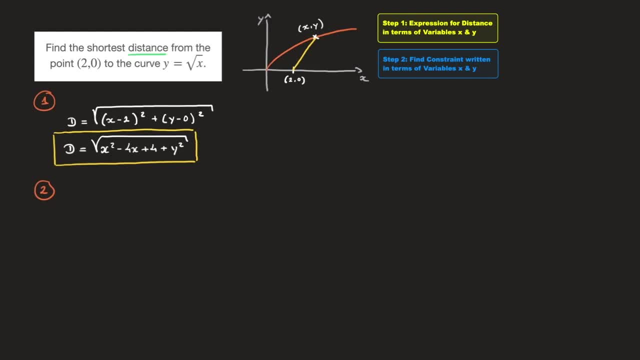 That's exactly how we write the constraint in this case. We just need to state that y must be equal to the square root of x, And that's the second step done. We now have the constraint written in terms of the variables x and y, So we move on to step three, And in step three we're. 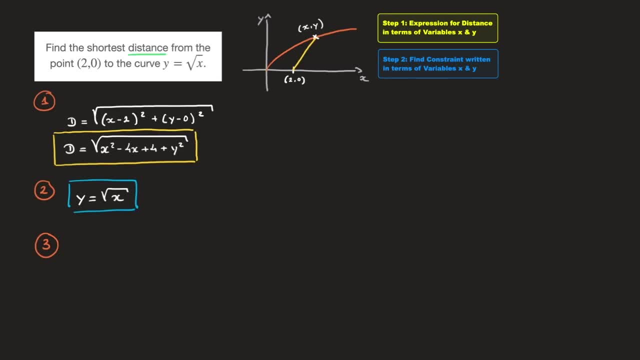 going to use the constraint we just wrote in order to eliminate one of the variables x or y inside the expression we wrote in step one. So that's the expression we just wrote. Now let's look at the expression for d here, Looking at the expression we have for the constraint. 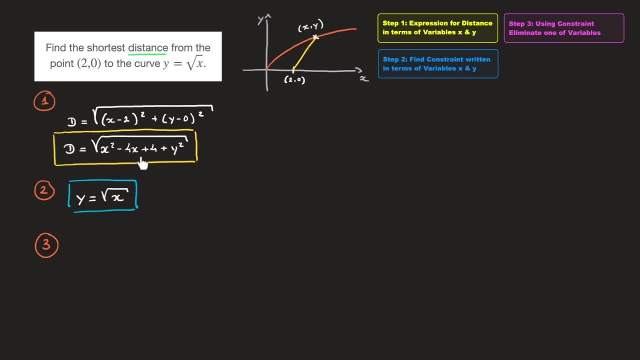 it seems easiest to replace every y we see inside the expression for d by the square root of x, So that leads to: d equals to the square root of x squared minus 4x plus 4, plus, in parentheses, the square root of x squared. Now, opening up this pair of parentheses, we have the square root of x. 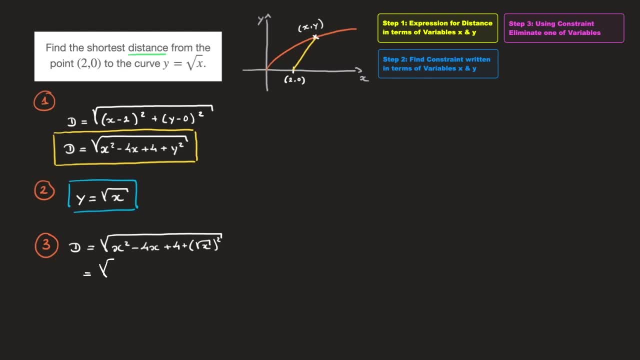 squared, which is just x, and then we have the square root of x squared, which is just x. So this becomes the square root of x squared minus 4x plus 4 plus x. And finally, simplifying, we can state that d is equal to the square root of x squared minus 3x plus 4, where all I've done 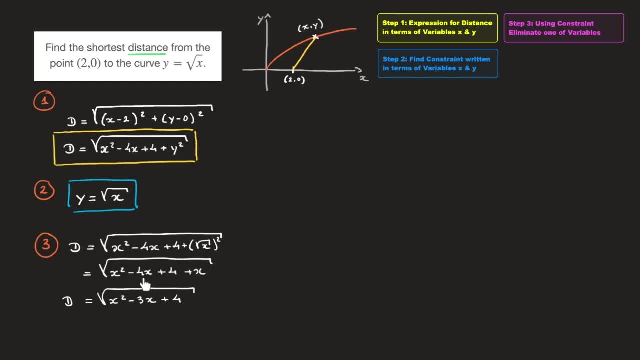 to get from this line of working to this one is gather the two x terms that we have here. That being said, that's the third step done. We now have an expression for the quantity we're trying to minimize, written in terms of one variable only, in this case x, And so, if we wanted to, we could actually say: this is a. 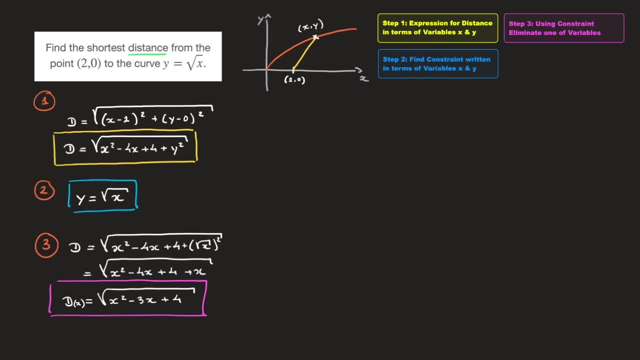 function of x, and we could write d of x right there. Next I move on to the fourth and final step, And in this step I'm actually going to optimize. In other words, for this case I'm actually going to find the minimum value of this function, And for that I use calculus. 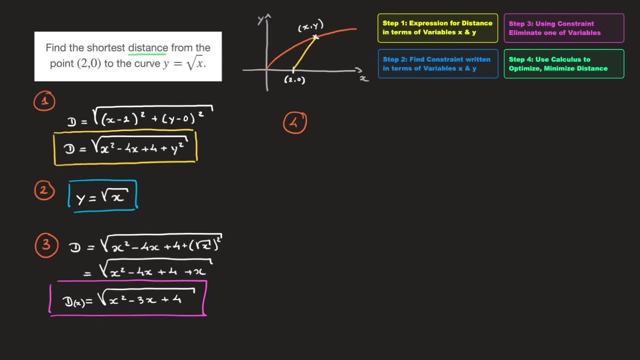 So, starting from the function we have here, which in fact you have the top, here we have d of x, which equals to the square root of x squared minus 3x plus 4.. The first thing we do is differentiate this function, And for that we use the chain rule. 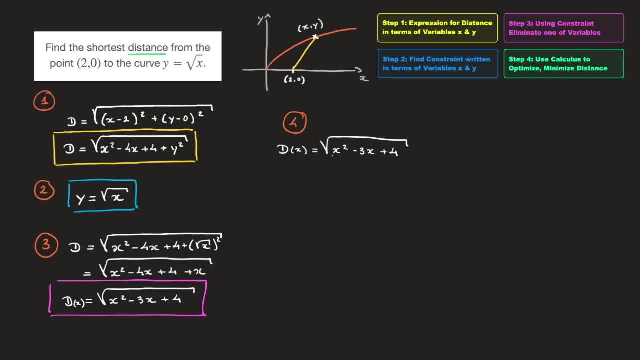 for differentiation. Indeed, if I call the inner function x squared minus 3x plus 4 u, then, using the chain rule, we can go ahead and state that the derivative of capital D with respect to x is equal to the derivative of capital D with respect to u times the derivative of u with respect to x. 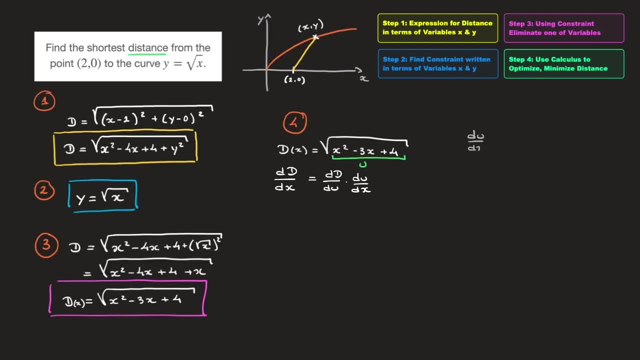 Now, on the side, here I can go ahead and do that working. I know that the derivative du dx I can find using the power rule. Indeed, I can state that that's equal to 2x minus 3.. And if I consider d as a function of u, I would write: d is equal to the square root of u And. 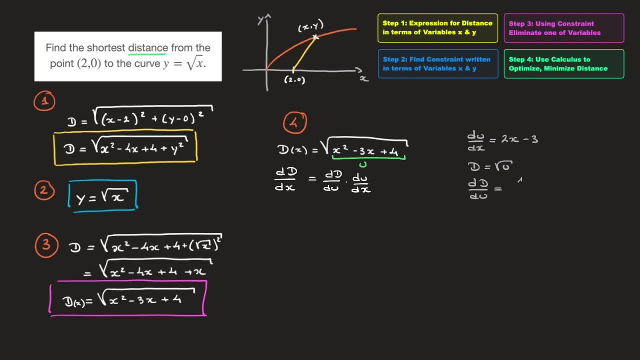 therefore, the derivative of capital D with respect to u is equal to 1 over 2 times the square root of u, And it's worth pointing out that, if you're unsure of how I'm getting from here to here, that derivative comes up very often and it's simply worth knowing off. 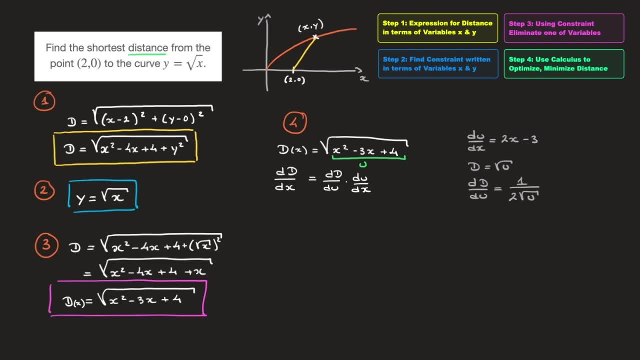 by heart And now that I've got the working out of the way, I can go ahead and state that that's equal to 1 over 2 times the square root of u times du dx, which we just saw, was 2x minus 3.. 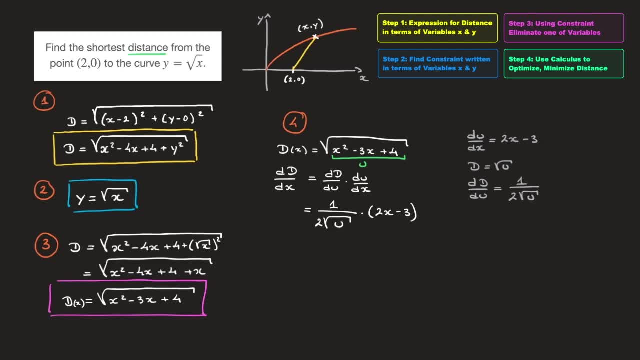 Now, multiplying this numerator by 2x minus 3 and replacing u by x, squared minus 3x plus 4, leads to the derivative of capital. D with respect to x is equal to 2x minus 3 over 2 times the square root of x squared minus 3x plus 4.. 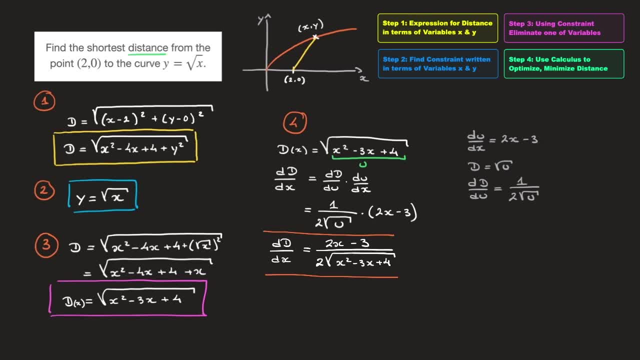 And in fact I'll go ahead and box that result. There we go. OK, now that we have the derivative to figure out where any maximum or minimum point occurs, we need to equate this derivative to 0.. In other words, we need to find any values of x at which the 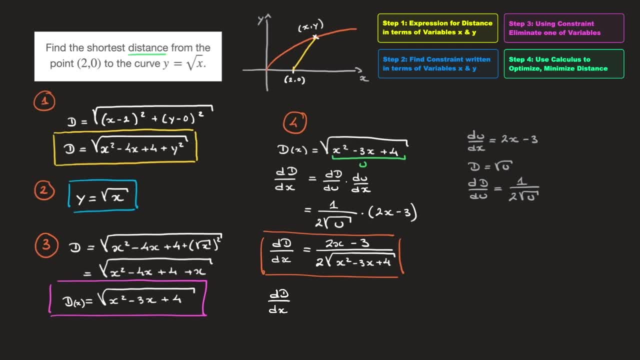 derivative of capital D with respect to x equals to 0.. And that is where 2x minus 3, over 2 times the square root of x, squared minus 3x plus 4, equals to 0.. Now to solve this equation. 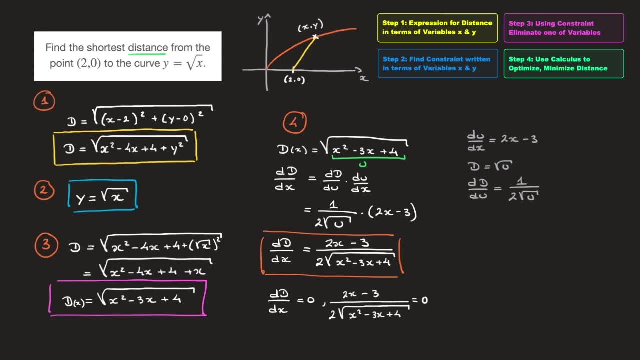 it's important to remember that the only way this fraction can equal to 0 is if the numerator equals to 0. In other words, solving this equation is the same thing as solving. 2x minus 3 equals to 0. And so adding 3 to both sides of this equation. 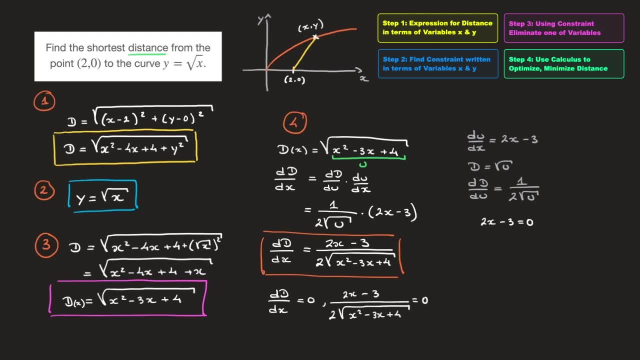 as well as dividing both sides by 2, we quickly find that x equals to 3 over 2.. And at this value of x, the function d of x reaches a stationary point. And so plugging this value of x into the derivative of x, squared minus 3 over 2 equals to 0.. And so plugging this value, 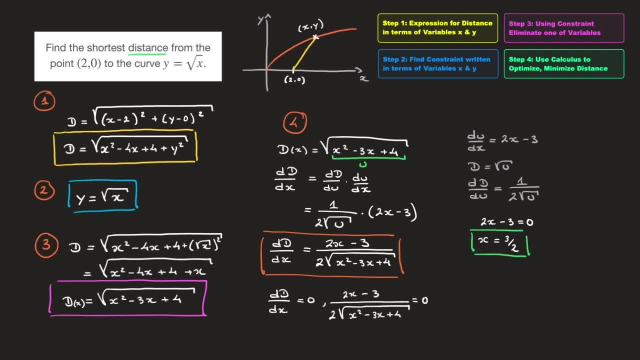 of x inside y equals to the square root of x- will give us the y coordinate, And that would be: y equals to the square root of 3 over 2.. And I'll go ahead and box that as well. There we go Now. the fact that the derivative equals to 0 at this value of x tells us that the point. 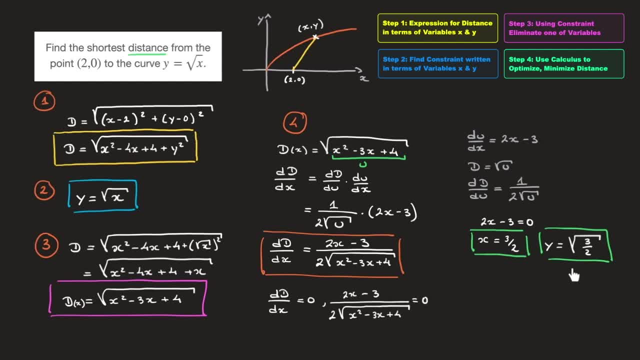 along the curve with coordinates 3 over 2, and square root of 3 over 2 is a stationary point. But how can we be sure that that stationary point is indeed a minimum? Well, first of all, it's clear that this stationary point cannot be a maximum. Indeed since this: 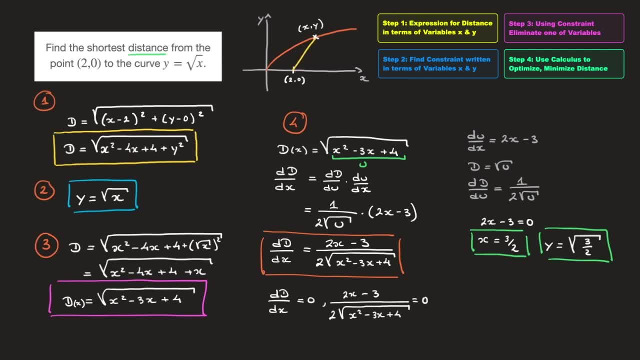 curve goes on forever. there's no limit to how long this line segment can get There, therefore can't be a maximum. This stationary point is therefore either a minimum or a horizontal point of inflection, But which of the two is it? Well, let's see. Let me start by adding this point on. 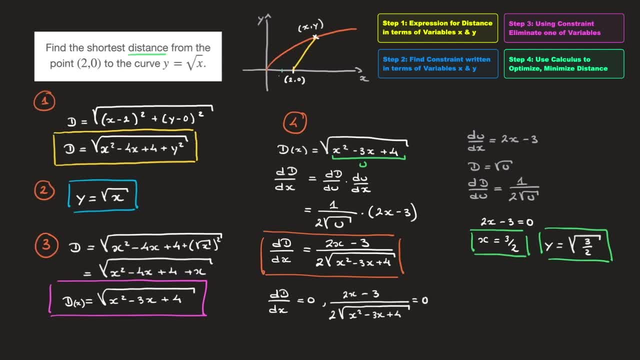 our curve. So that's the point- whose x coordinate is 3 over 2, and I'll say that's here- and whose y coordinate is the square root of 3 over 2.. So that's the point we're dealing with, right here. 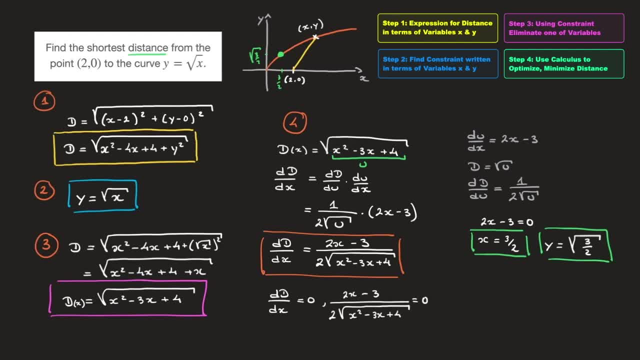 And so the distance from that point to the point with coordinates 2, 0 would correspond to the length of the green line segment I'm drawing right now. Now, since, beyond a certain point, it's clear that the distance from the curve to the point with coordinates 2, 0 gets bigger. 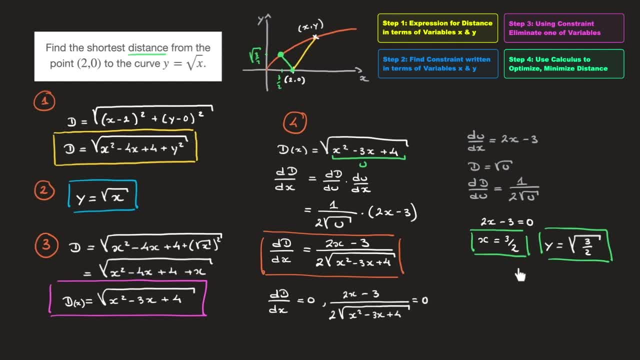 and bigger and bigger. If this stationary point corresponds to a horizontal point of inflection, it must correspond to an increasing horizontal point of inflection, And that would mean that the shortest distance from the curve to this point would be the distance from its starting point at 0,, 0 to the point. On the other hand, 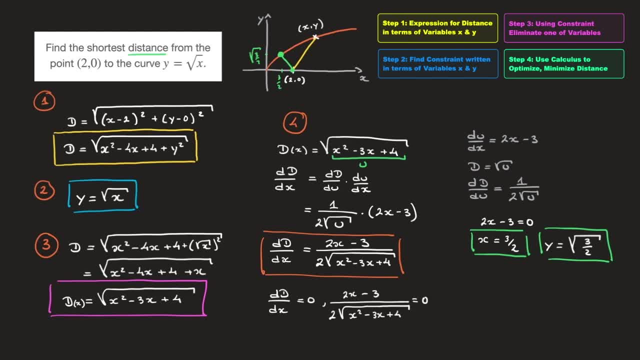 if this stationary point corresponds to a minimum, it would mean that the length of this green line segment is the shortest distance. So which one is it? Well, to answer that question, I like to study the sine of the derivative, And for that I'll make a small sine table on the far right-hand. 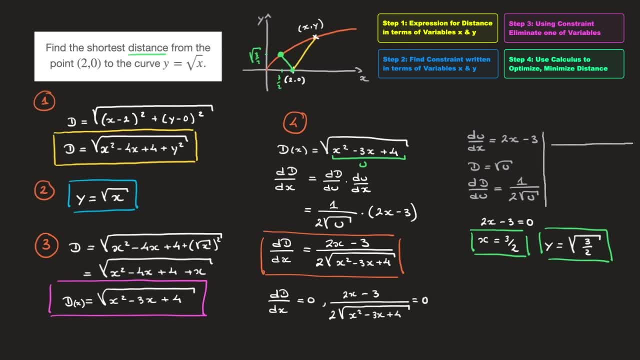 side here. So, let's see, I'll have a top row here That will be for the different values of x, And I'll make a small sine table on the far right-hand side here. So, let's see, I'll have a top row here That will be for the different values of x. 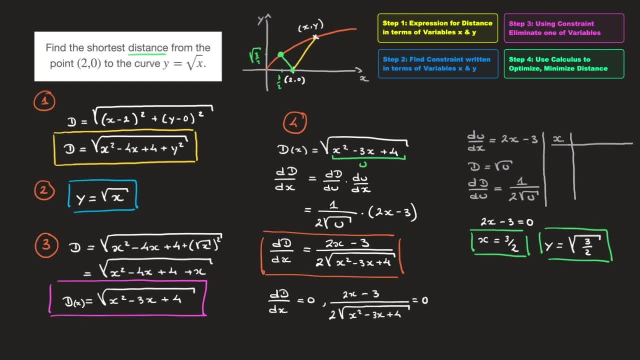 And I'll make a small sine table on the far right-hand side here. So let's see, I'll make a small sine table on the far right-hand side here And I'll construct a column like so: And in the second row of this table I'm going to study the sine of this derivative. 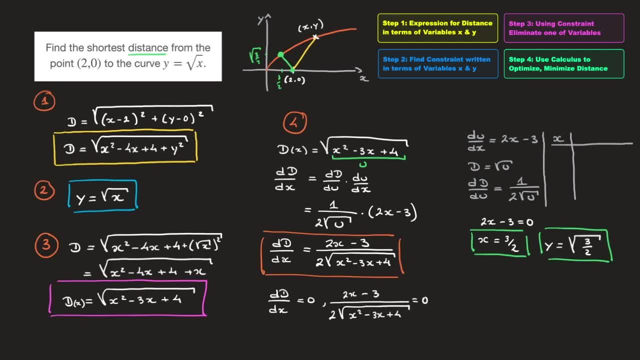 That is, figure out where it's positive, negative and zero. Now, looking at the derivative we have here, since the denominator we have here will always be positive, the sine of this derivative will depend entirely on the sine of the numerator. So that's the sine of 2x minus 3.. So all I really have to study here is the sine of 2x minus 3.. 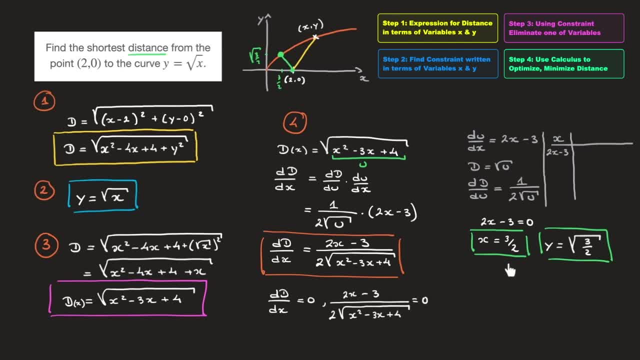 So all I really have to study here is the sine of 2x minus 3.. Well, we know that it's equal to zero when x equals to 3 over 2.. And so I can add that value of x on the top row here. That's 3 over 2.. 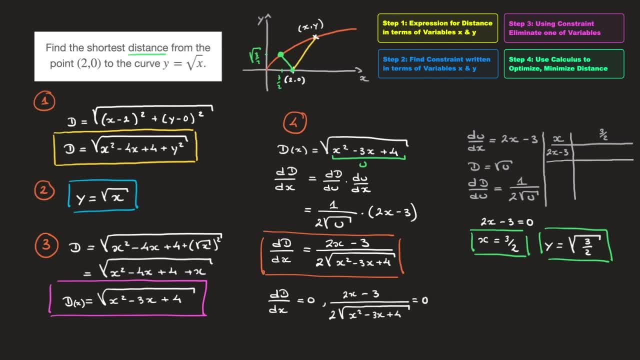 And add that value of x to x minus 3, and therefore the derivative is equal to zero. But what about the sine of the derivative on either side of that value of x? Well, let's see For x values less than 3 over 2, and in fact, to be more specific, 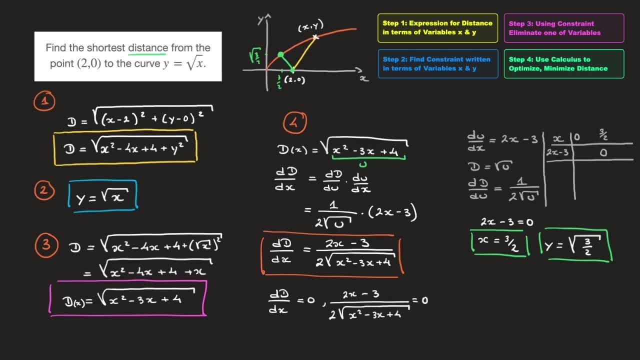 we could say for x values between 0 and 3 over 2, 2x minus 3 is 0.. 2x minus 3 will be negative And to convince yourself of that you can plug in any value of x between 0 and 3 over 2. 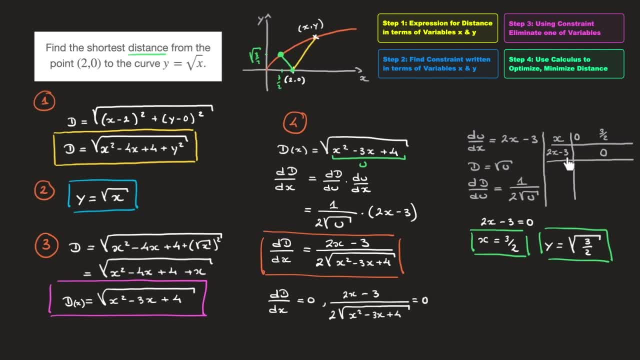 inside 2x minus 3, and you'll get something negative. For instance, to make our life easy, let's say we took x equals to 1, then this would be 2 times 1,, which is 2, minus 3,, which is negative 1.. 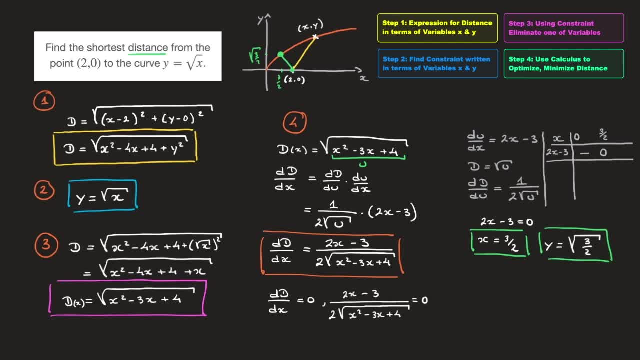 And that's negative. So we can write a negative sign here For x values greater than 3 over 2, so on the right hand side here, 2x minus 3, and therefore the derivative will be positive. And again to convince yourself of that, take any value of x greater than 3 over 2,. 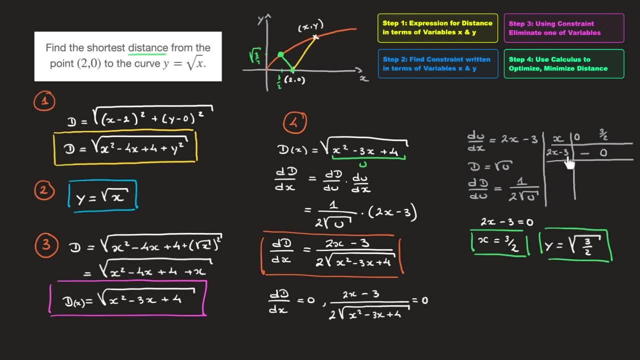 for instance, take 2, and plug it inside 2x minus 3.. So for x equals to 2,, that would be 2 times 2,, which is 4, minus 3,, which is 1.. And since that's positive, we can write a plus symbol right here. 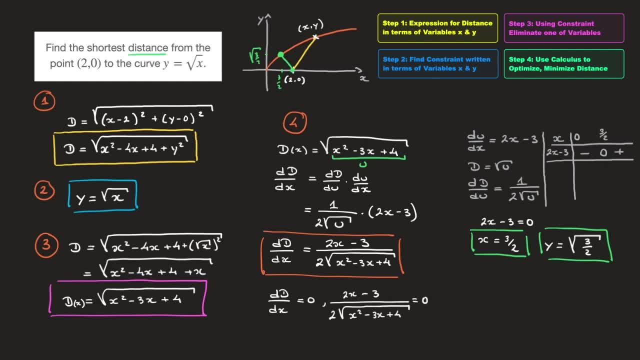 And so we now know that on either side of this stationary point, the derivative goes from negative to positive. Consequently, the function d of x must be going downwards. when the derivative is negative, it reaches a minimum point and then goes upwards when the derivative is positive. 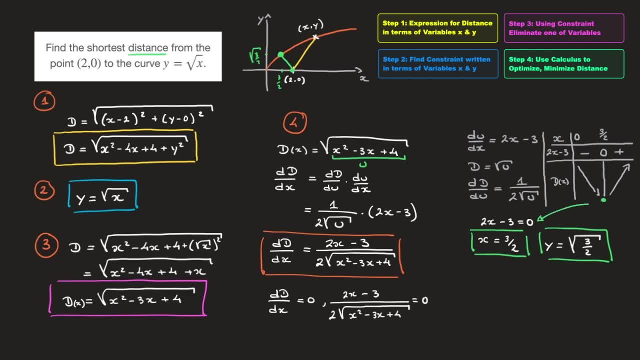 And this minimum point can only correspond to the stationary point whose coordinates we just found, which allows us to conclude and state that the shortest distance from the point with coordinates 2, 0 to the curve is the distance from the point to the point we just found. 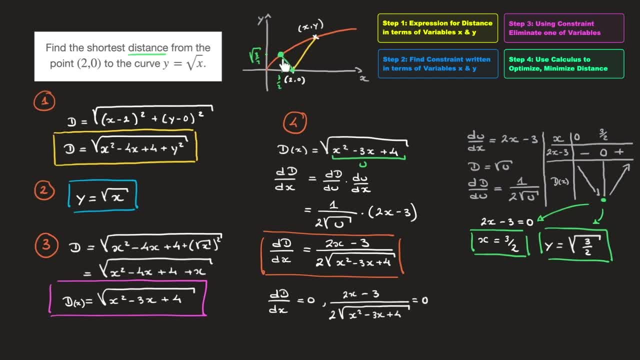 And so all we have to do now is calculate the length of this line segment, And to do that, I'll go ahead and use the expression that I boxed here earlier on. All I need to do to calculate the distance is replace every single x, I see, by 3 over 2.. 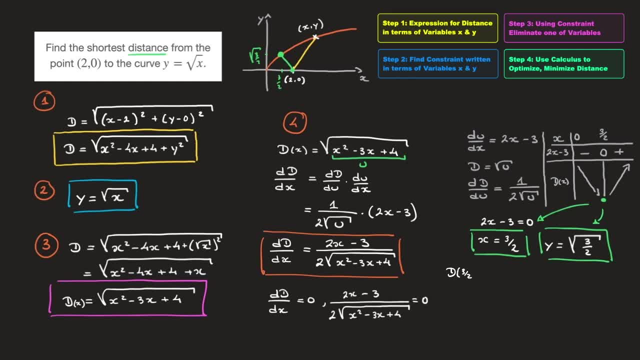 So let's see that would be d of 3 over 2, and that's equal to the square root of 3 over 2 squared, minus 3 times 3 over 2,, plus 4.. Now, since 3 over 2 squared leads to 9 over 4, and 3 times 3 over 2 leads to 9 over 2,. 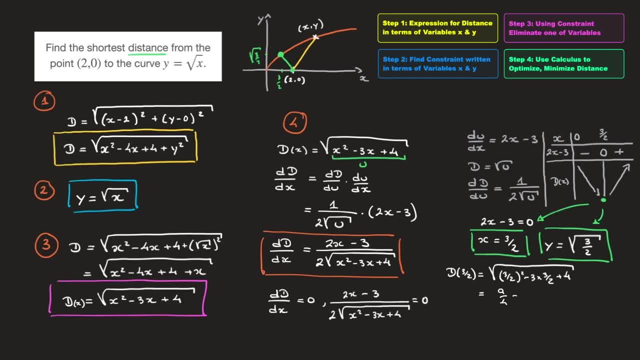 this becomes 9 over 4 minus 9 over 2 plus 4.. And all of that's under a square root. there we go Now. 9 over 4 minus 9 over 2 is negative. 9 over 4,. 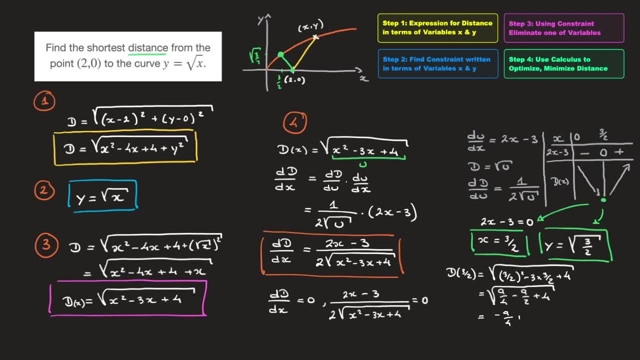 so this equals to negative 9 over 4 plus 4, and again that's under a square root. And finally, since we have the distance from the point to the point, the distance from the point to the point, Since 4 is the same thing as 16 over 4, we have negative 9 over 4 plus 16 over 4, which 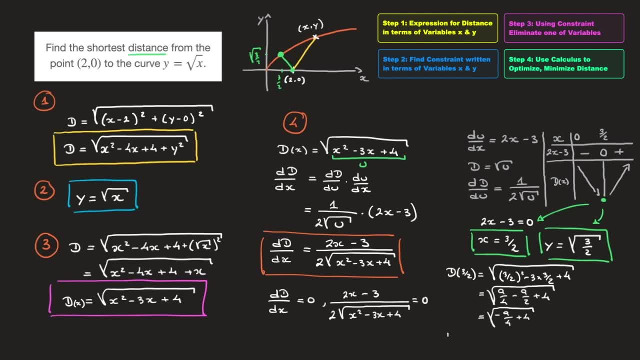 is 7 over 4.. And so we can state that the shortest distance from the point with coordinates to the curve is equal to the square root of 7 over 4., Which we could also write as the square root of 7 over 2.. 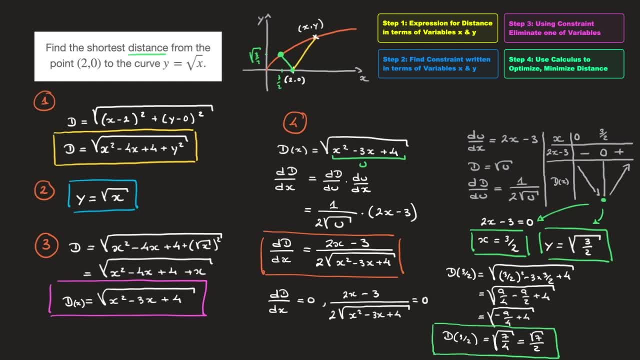 And that's the final answer. We've just solved a must-know type of problem when studying optimization for calculus, And that's it for this tutorial.